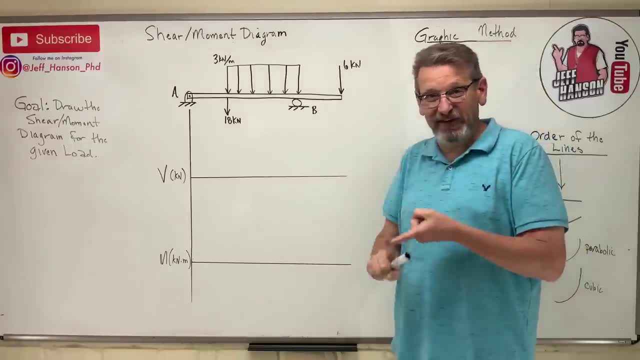 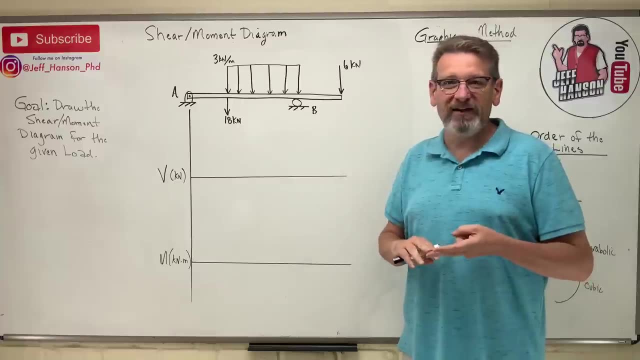 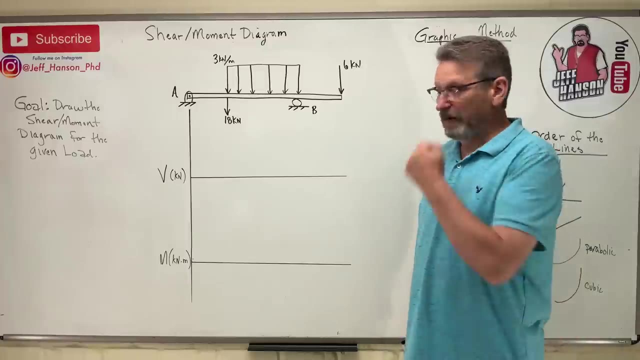 diagrams. We've been talking about internal forces, M and V, right? Well, what happens if I ask you what is the value of V and what is the value for M? instead of at a single point on this beam, maybe here, What is it at every point on the beam? Well, the only way to do, this is when you ask a square. I'm just going to wrap theref and repeat what I think it's meant to be. If you're interested in an introduction on entire forces, best use the America並 tenir, and you're left with a square. 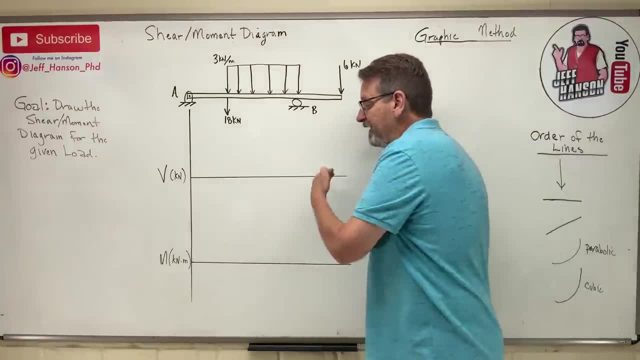 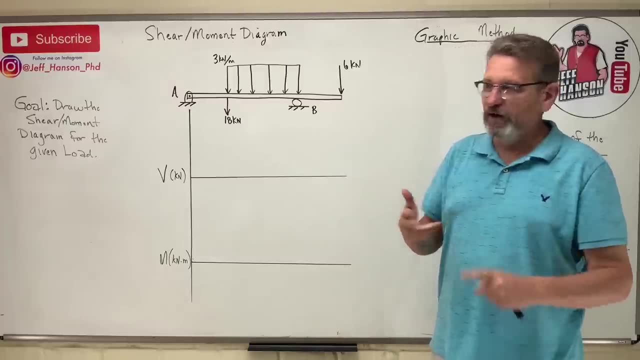 that is, to graph the V right And then graph the M for every point on the beam, And that way you could ask me what is the value of V, What is the value of M for any point on the beam, And where. 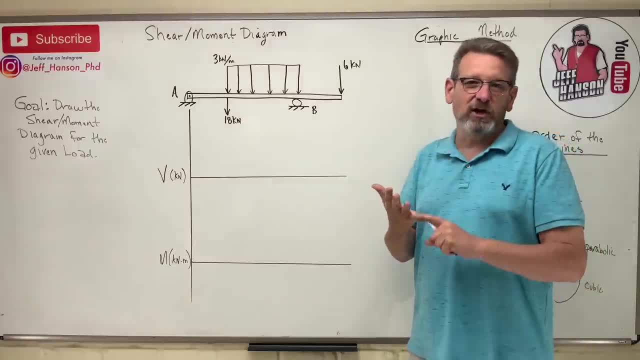 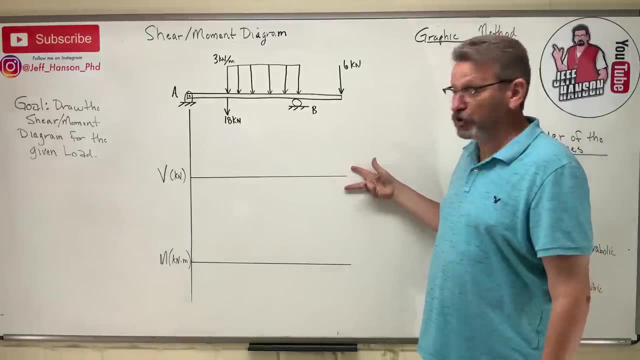 is that going to become important? Well, when you get to, especially when you get to solids right, There's going to be some stuff, like when you're designing beams and you're going to need to know to design for the very biggest shear force on that beam. So you're going to need to know where. 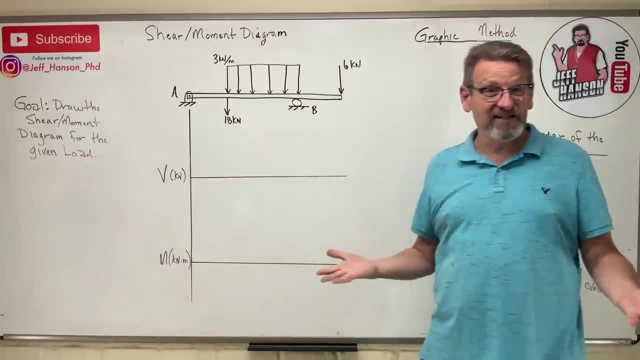 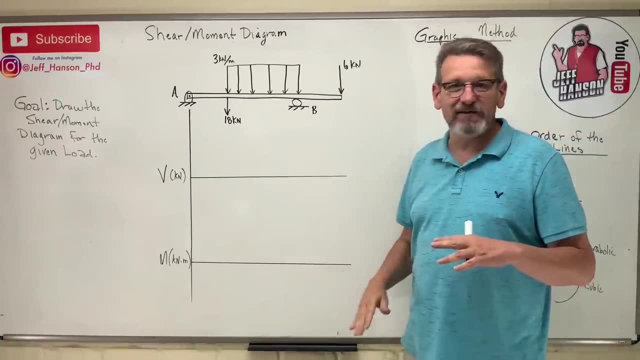 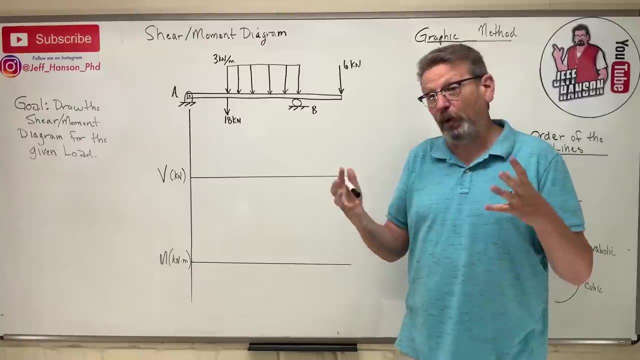 does that occur? Well, if I plot all the points, I can see where it occurs, right. Same thing for M for beam bending: right, We use bending moment, which is what this is, And if I knew where that maximum bending moment occurred, I knew what. I would know how to design my beam to support that. 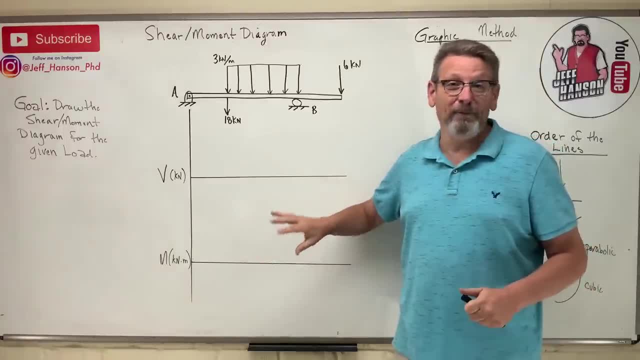 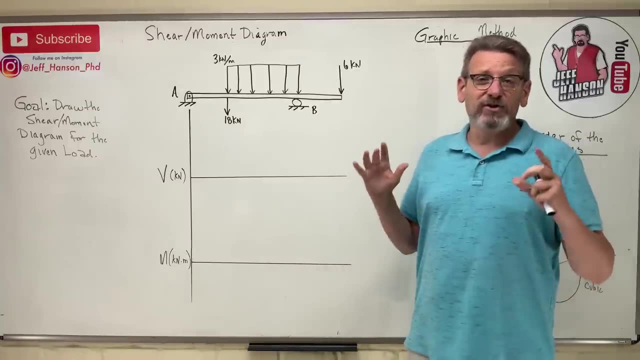 load. So it's important to know what is the absolute max bending moment on a beam, So we plot that and then we can see exactly where that maximum is Okay. So there's a few tricks that you need to know. First of all, you need to know what the maximum bending moment is, So you need to 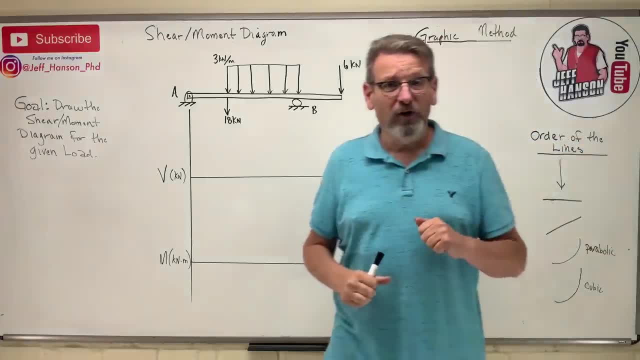 know what the maximum bending moment is. So you need to know what the maximum bending moment is, So you need to know to do shear moment. diagram problems And number one: we'll start off with this. Okay, When you do these problems, you need to make sure that you start off with this at the top of your 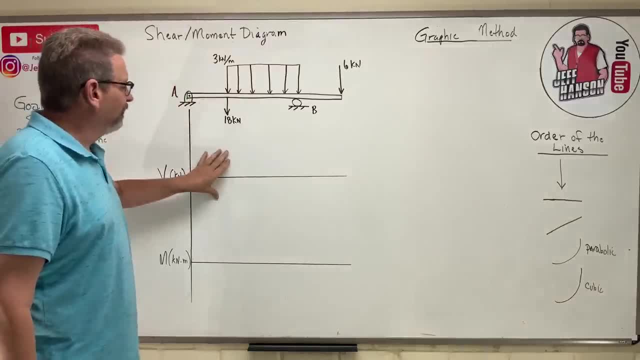 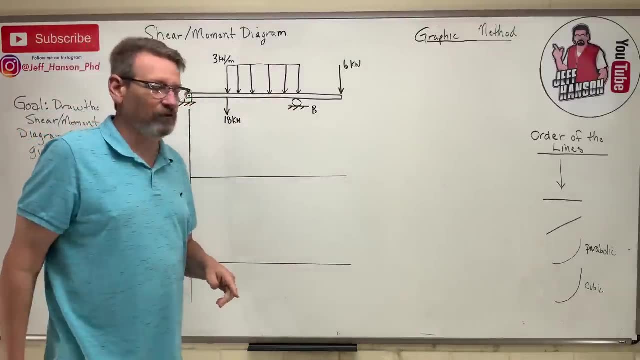 page in your notes, because this graph is related to that graph is related to that graph, So they need to go kind of one under the other. You can't do this one on the next page. It makes no sense because it is totally based on what's going on here. Okay, And they're related to each other in. 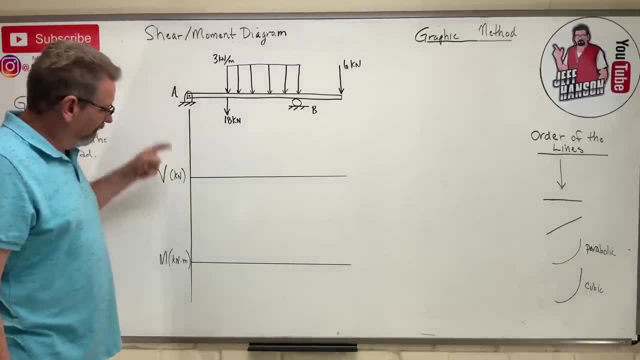 this way. This graph is the integral of that graph, So you need to know what the maximum bending moment is. Okay, So you need to know what the maximum bending moment is. Okay, So you need to know what the maximum bending moment is. Okay, So you need to know what the maximum bending moment is. 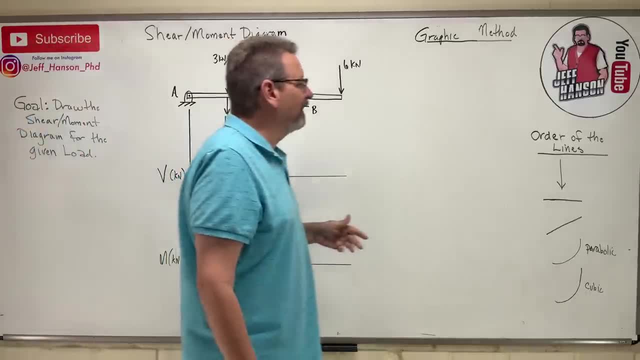 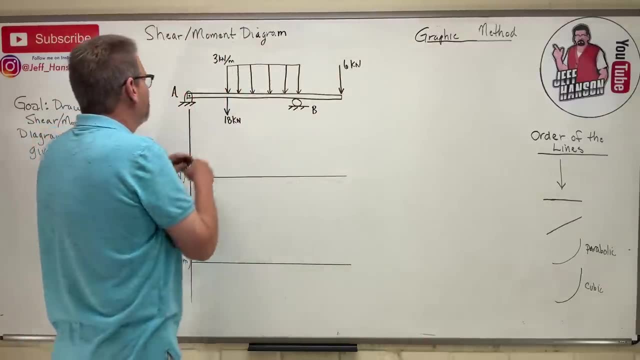 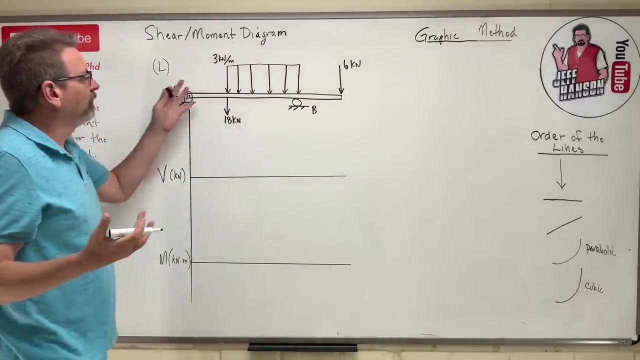 This graph is the integral of that graph. So if I have something like this, I've come up with what I call the order of the line. So as we go down the graph- you know this- I call the load curve. right, This is the given graph that you're going to have to do, or the given load to a certain beam. 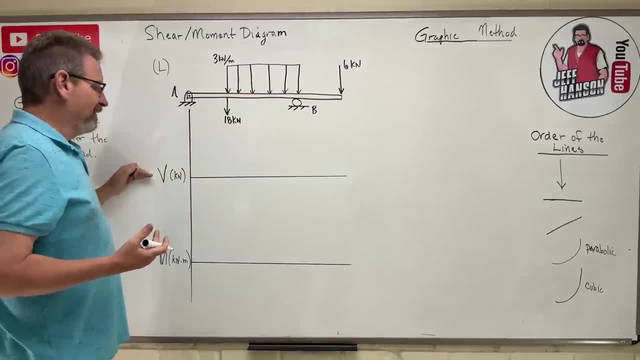 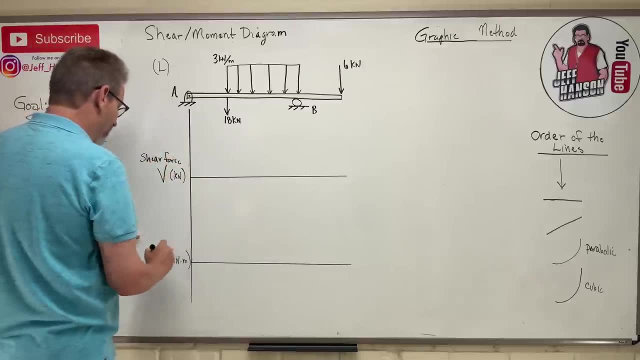 that you're given And from that you're going to find the shear force. This is for shear force. We already talked about what that is Okay. And then this down here is your bending. That looks like an O. It's not bonding moment, but that's bending. 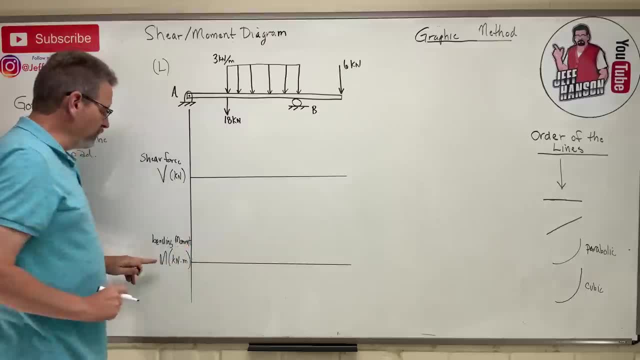 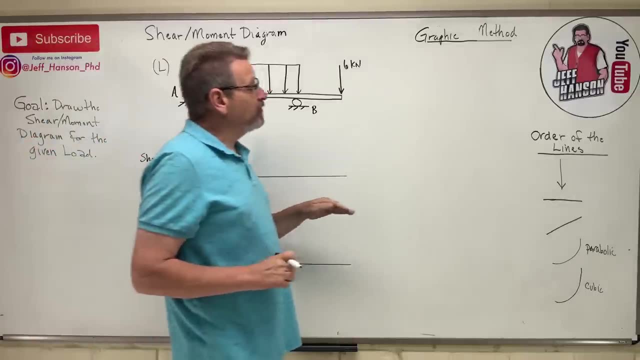 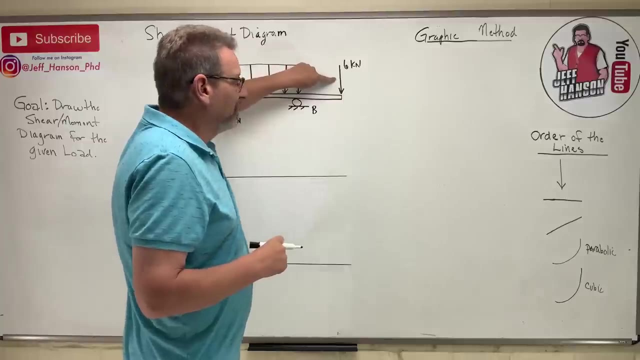 moment. Okay, This is your bending moment. This is your shear force. Okay, Like I said, this is the integral of that. This is the integral of that. So, as you go down those line, shapes are going to change. So if you have a concentrated load on the first graph, like here, the next, 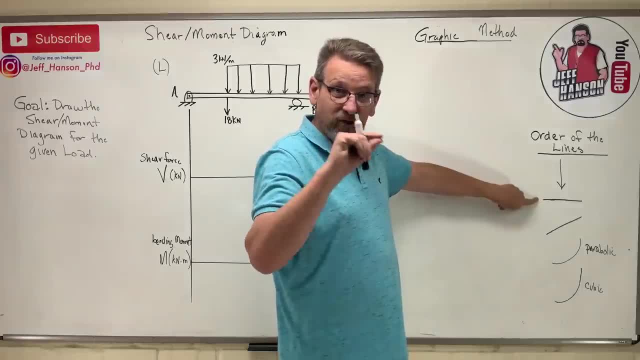 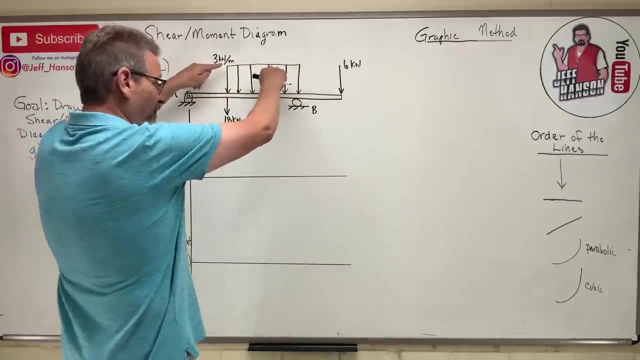 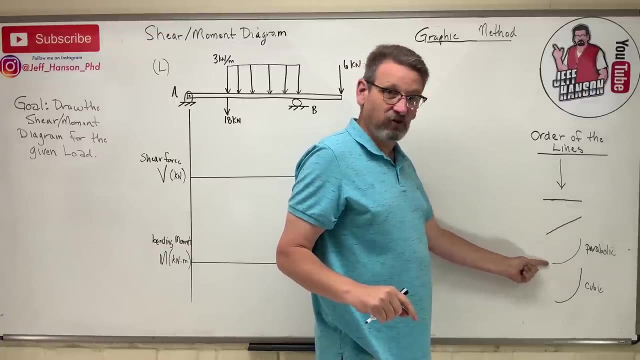 graph down in that area is going to have just a straight, a straight horizontal line. Okay, If I have a straight horizontal line, like I do right there, then the next graph down is going to have a slope. If I have a slope, the next graph down is going to be parabolic. If I 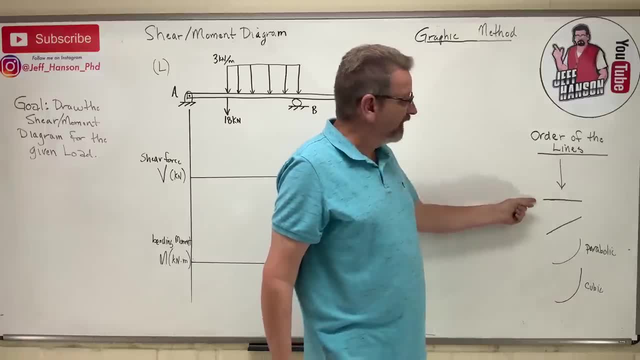 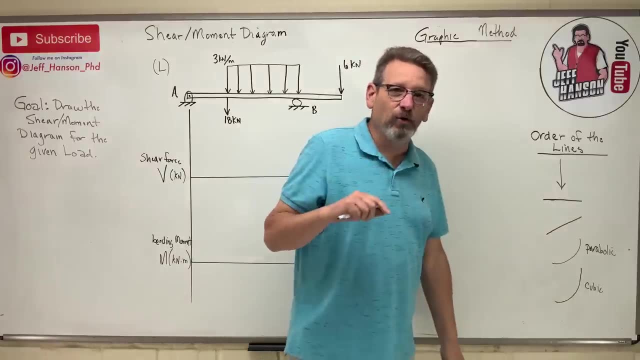 have a parabolic. the next because- and here's how it is Like, this one right here is like: y equals five, right, That's what it would graph like, just straight line, right? Okay, What's the integral of y equals five? That would be five x, right? How do you graph five x? Well, it's going. 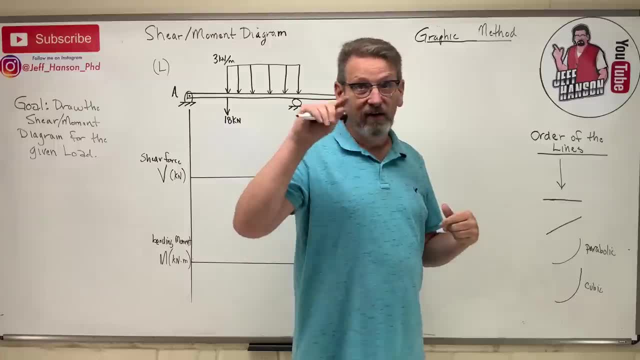 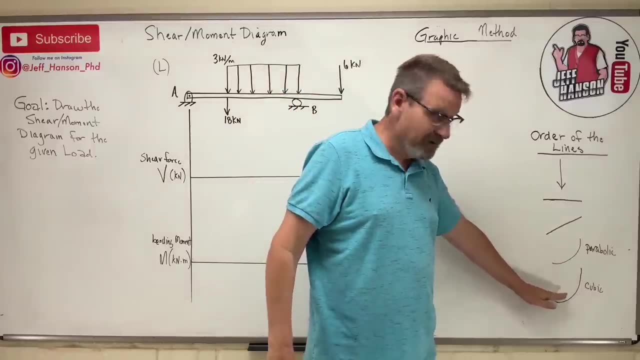 to have a straight horizontal line. So if I have a straight horizontal line, like I do right there, slope like this: Okay, What's the integral of five x? That would be an x squared, right. So that's parabolic. Integral of x squared would be x cubed- That would be cubic, right? So that's how those? 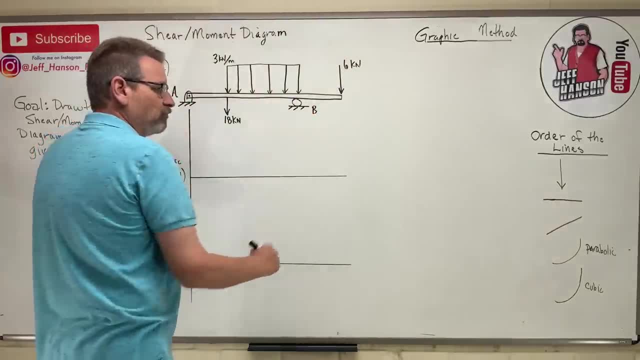 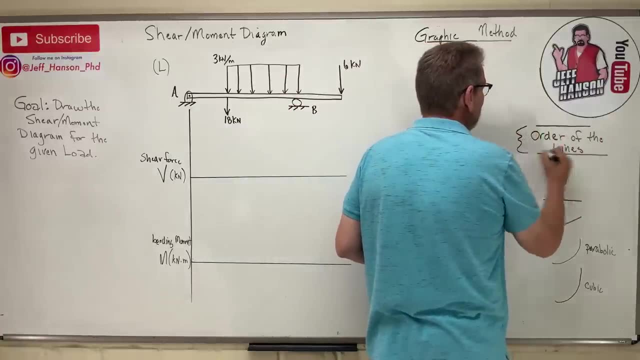 lines progress as you go down these graphs And so, if you remember the order of the lines, I call it this. don't look for this in the book, because I totally made this up, Okay, So don't look for that in the book, but the order of the lines: Okay, And it just kind of tells you what the next. 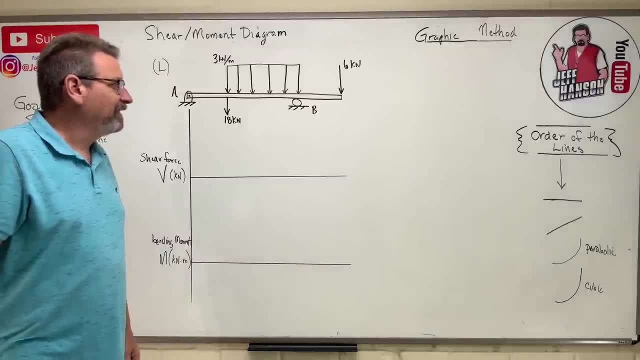 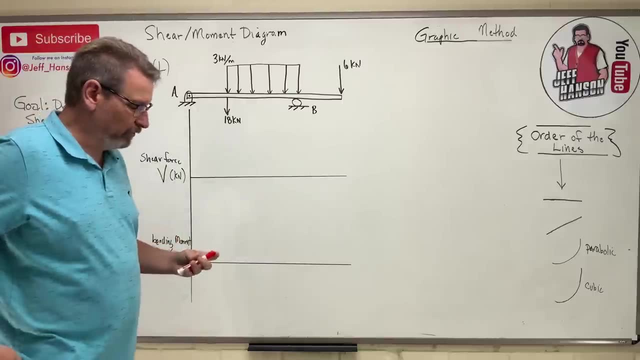 graph down is going to look like: Okay, Okay. Now this is going to start out like every other problem so far in the last two chapters, in that the first step that you have to do is you got to find global equilibrium. Okay, So for here, global equilibrium, what do we got? We got a pin. 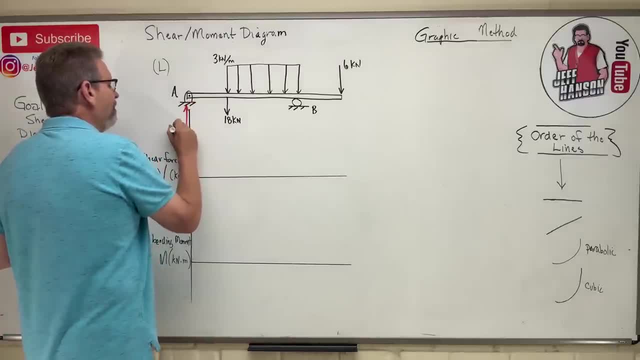 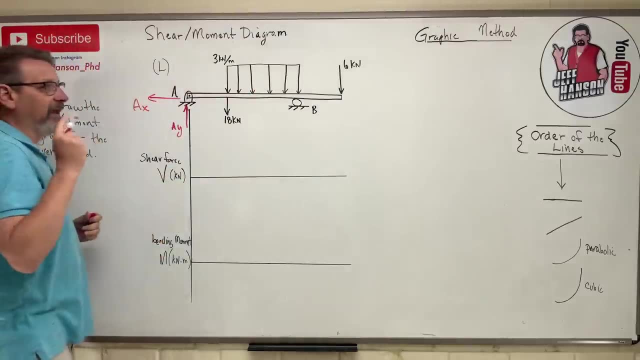 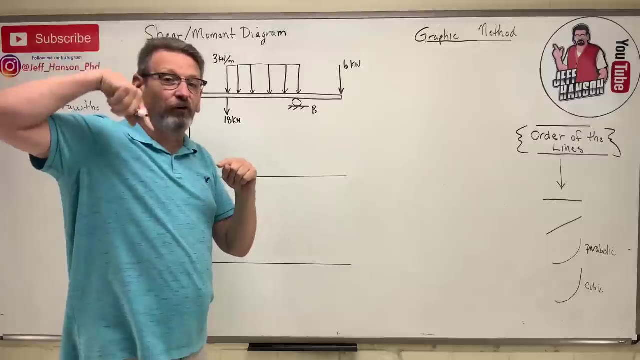 connection over here. So we're going to have an ay and we're going to have an ax. Now there are no forces in the x direction, And if you ever have one, let's say there's six on here. instead of going straight down was going at an angle. We're only interested in those vertical forces, So we 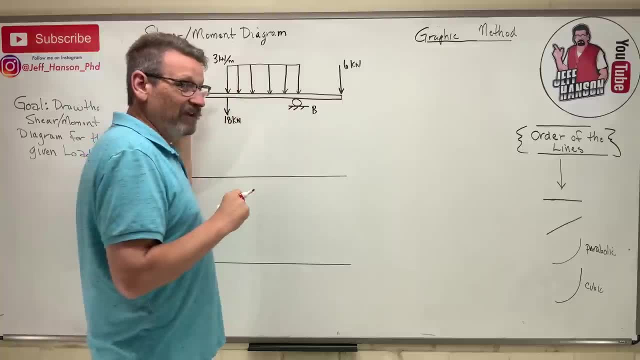 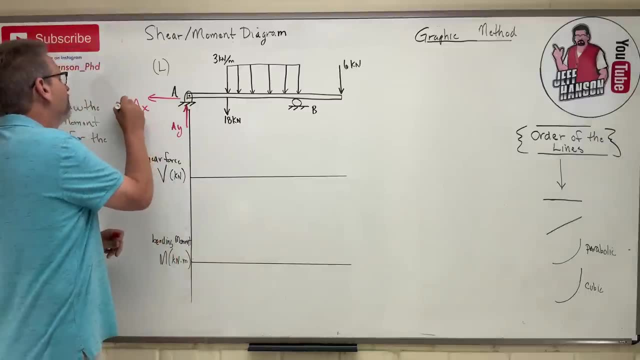 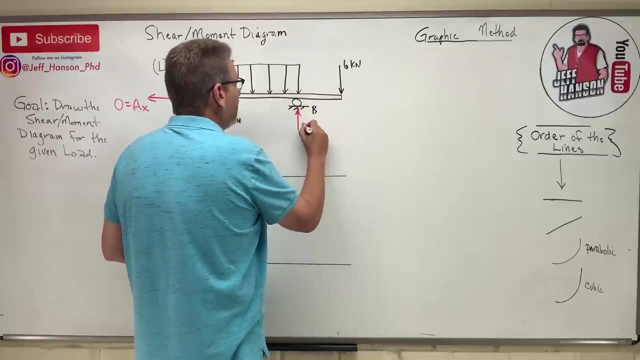 would just get the vertical component. We're not interested in things that are in the n direction for our internal forces, because there's no n graph, It's a, v and m graph, Okay, Okay. And then over here at b: okay, we'll have a by. Okay, It's a roller. Oh, and one more thing, Let's turn this. 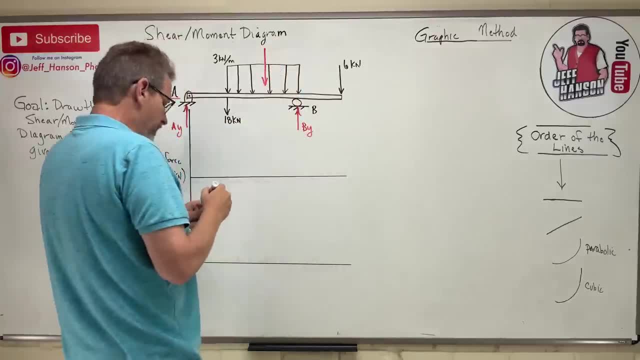 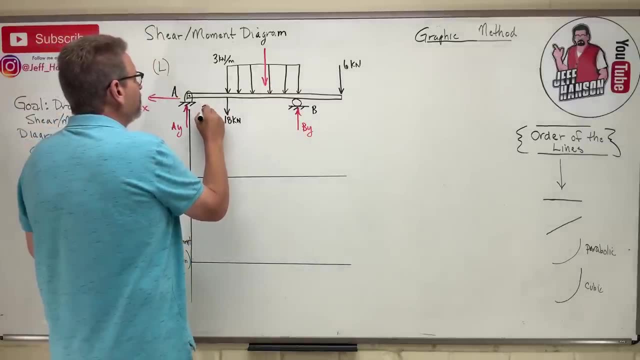 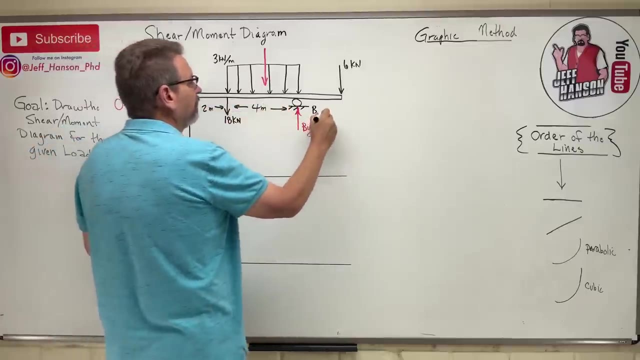 distributed load into a concentrated load. Dr Hanson, you didn't give us any dimensions. Oh no, Let's make them up. Okay, This looks like two meters, And then that looks like four meters, And then this one over here- again two meters. Okay, How's that? I just made that up. 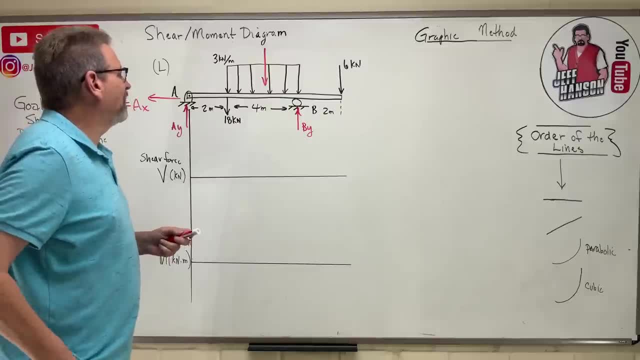 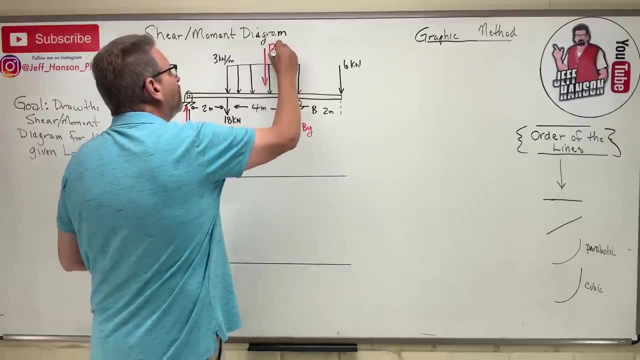 but we can do that, We have the power. Okay, So let's see three kilonewtons per meter. over four meters, That would be the same as 12 kilonewtons. Right And again. you just look at the area of. 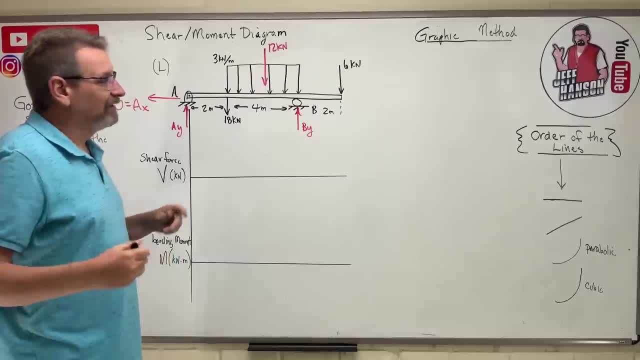 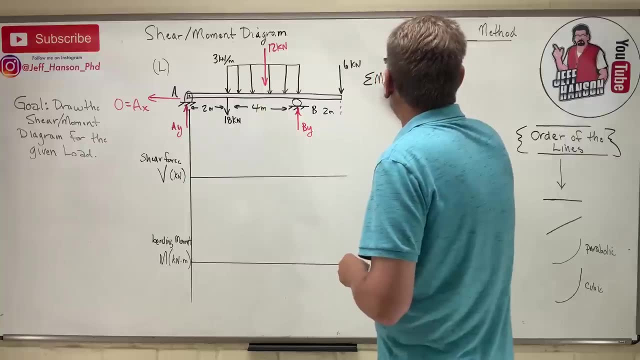 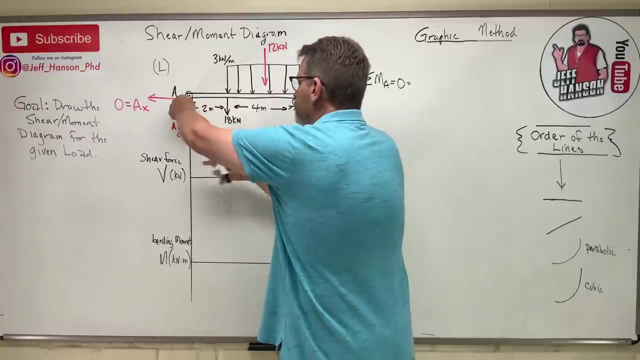 that shape there. Okay, So we got what we need. Let's find global equilibrium. Let's take a moment at a. Okay, Summing the moments at point: a equals zero. equals what? Okay, I've got this 18, which rotates me negative, So minus 18.. I'm so far away. Two: 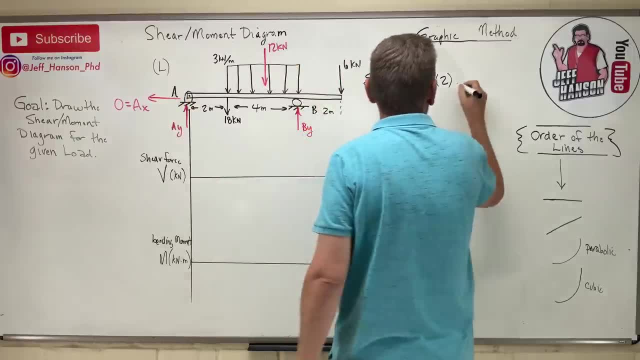 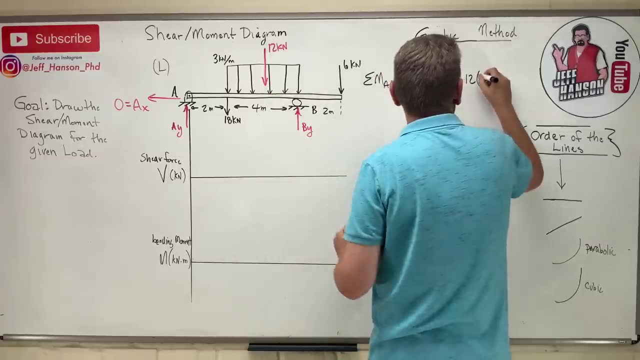 And then I've got this 12, which rotates me negative 12 minus 12 times. how far away is that? It's two And it's in the middle of this four. So two plus two more, That would be four. 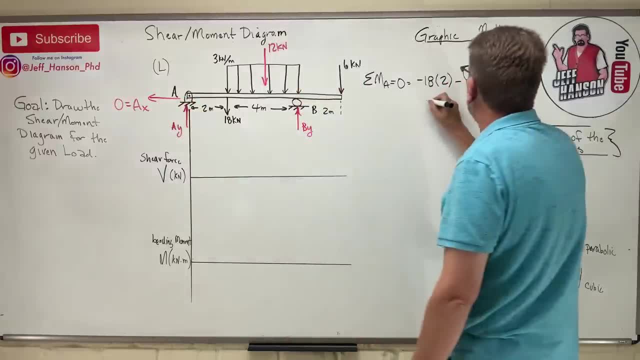 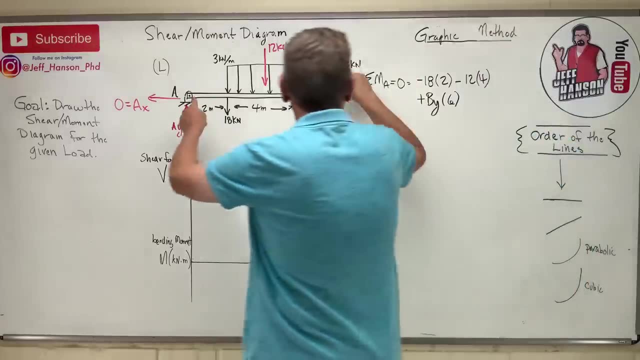 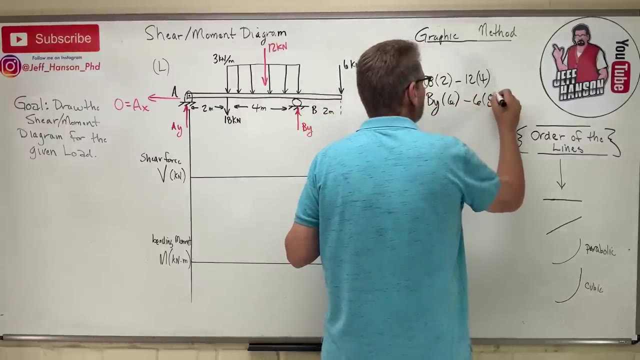 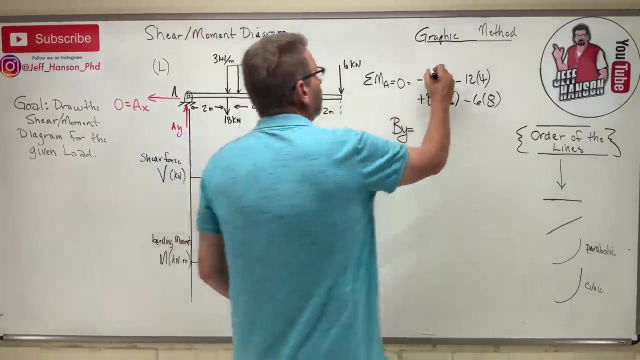 And then by rotates me. Oh, that's positive. So plus by times six. And then the six over here rotates me negative. So minus six times eight, Right, Okay, And so there by is equal to drum roll. please, Let's see, That's 36.. That's 48.. That's 48.. 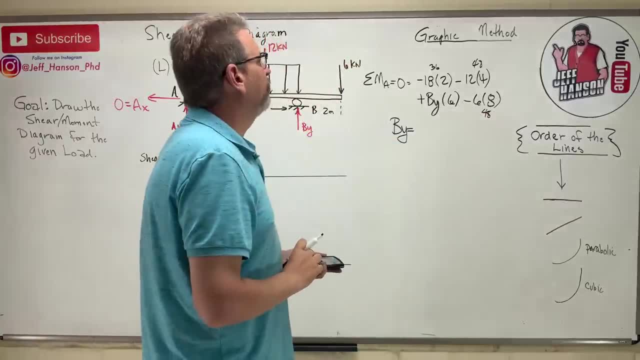 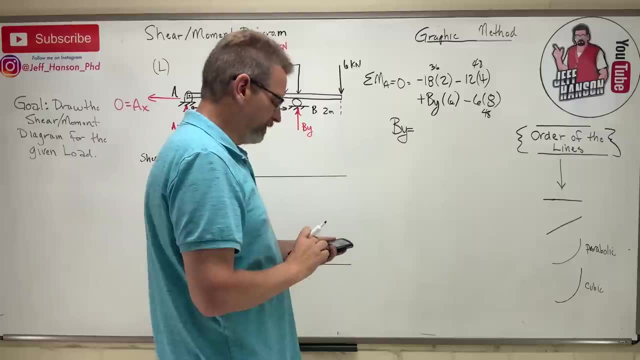 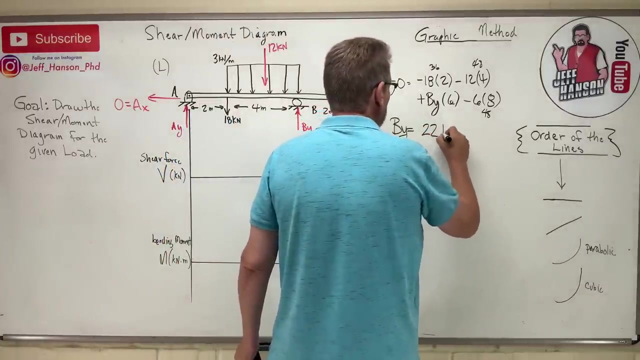 48.. 48, 48 is 96.. 96 and 100. And that's 132, isn't it Clear? Clear 96 plus 36. 132.. 32 divided by six equals 22.. So BY would be 22 kilonewtons. Okay, So that's you. You're 22. 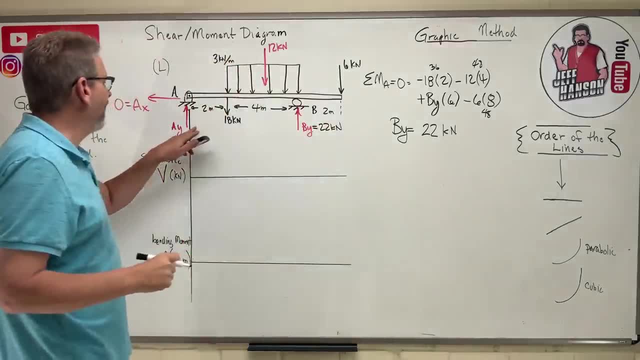 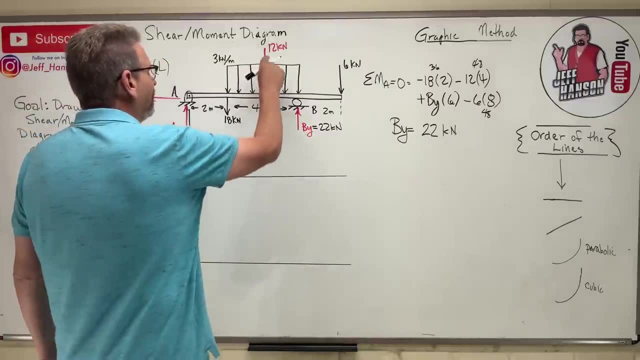 kilonewtons. Okay, And then, and then AY over here, Remember, the up stuff's got equal to down stuff. So what do I have going down? I got: 12 plus 18 is 30. Right Plus six more is 36.. 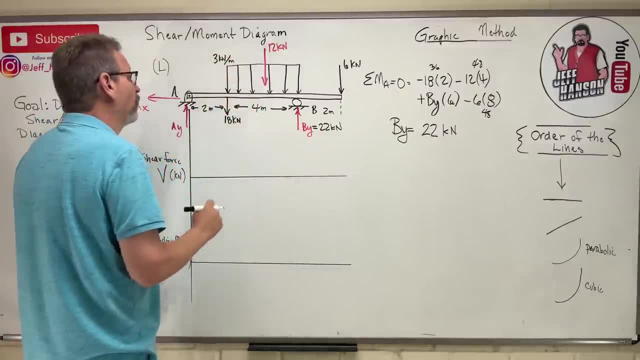 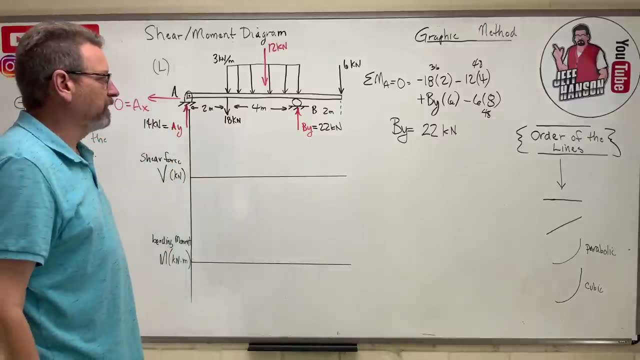 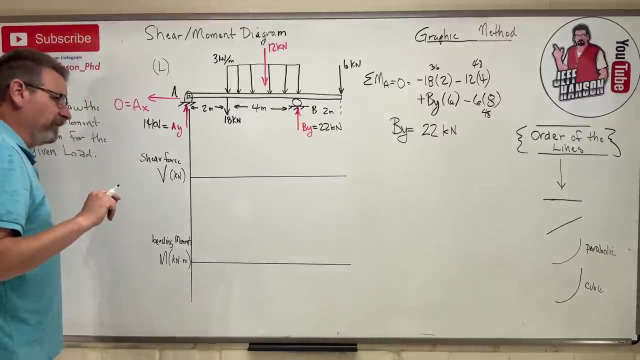 At 36 going down, I got 22 going up, So I need 14 more, don't I? Okay? There you go. So now we have our global equilibrium. That's step one done, Okay. The next thing we need to do, and if you do this on a digital homework, the first thing I have you do: 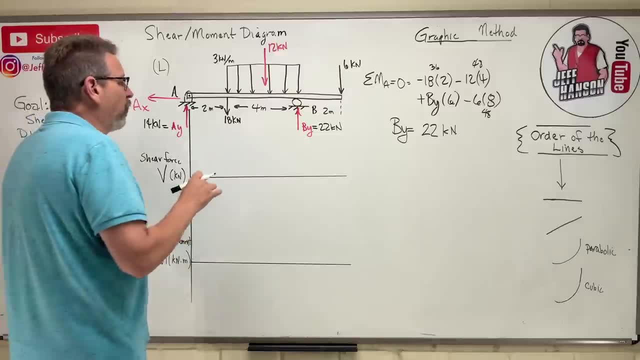 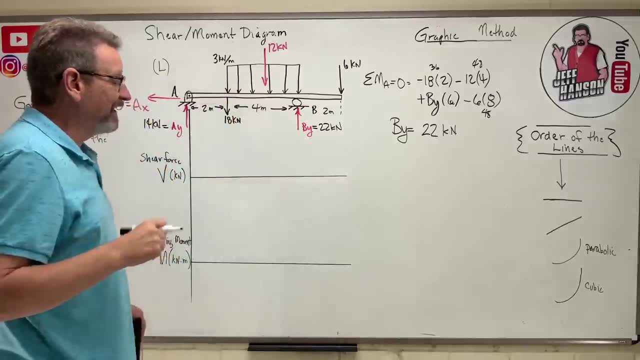 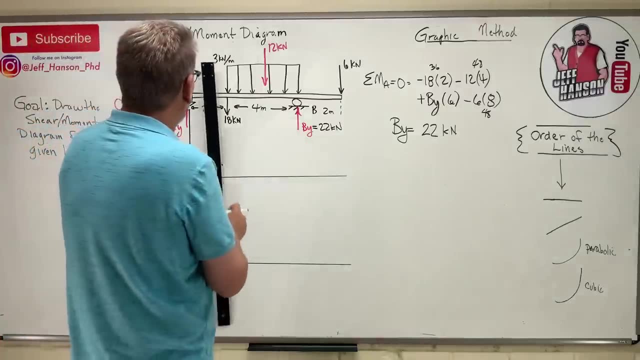 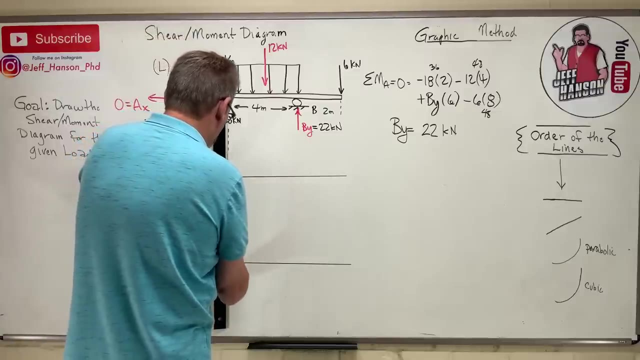 And we call those discontinuities And I just say, let's draw us a line everywhere. we think something interesting is going to happen. So I think something interesting is going to happen here. Okay, And these are called my discontinuity lines. Okay, I think something interesting is. 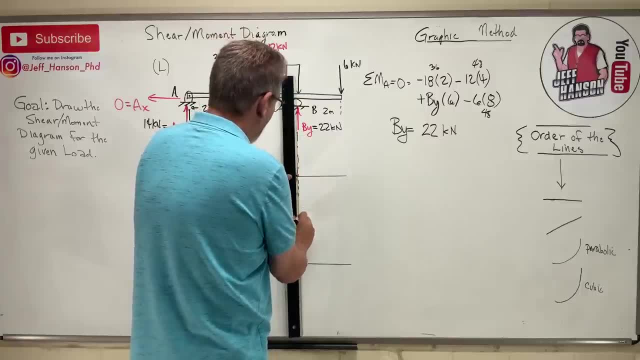 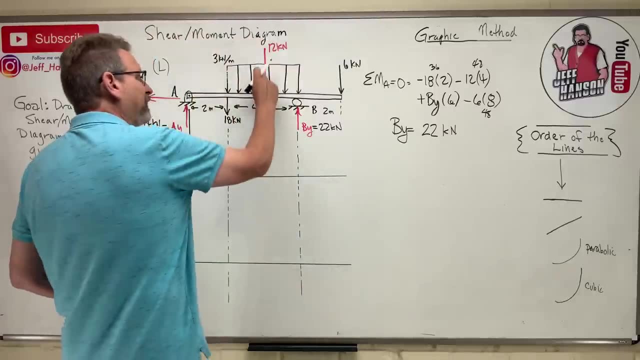 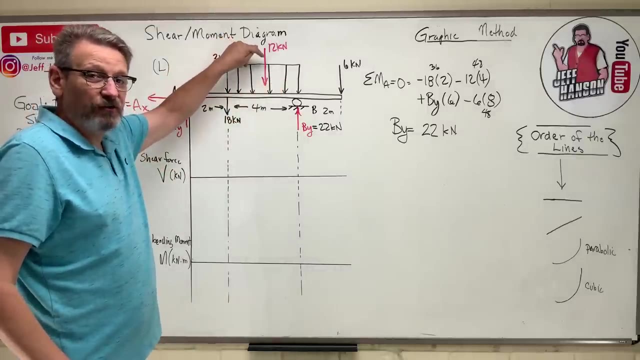 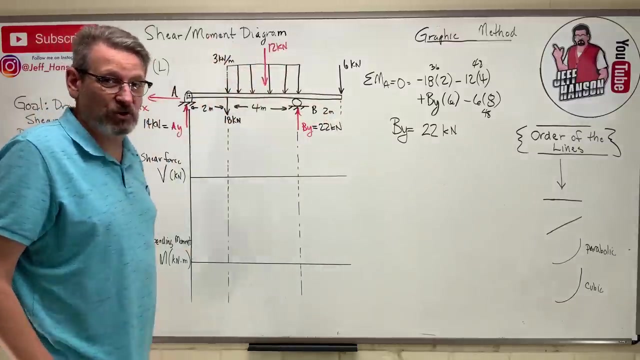 going to happen here. okay, now, i did not put anything here. this is a distributed load. it is not a concentrated load. we change it to a concentrated load only to help us find global equilibrium. after that, forget about it. it's got to go back to a distributed load because it is a distributed. 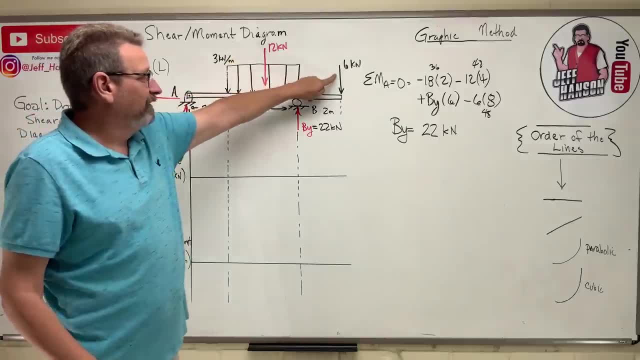 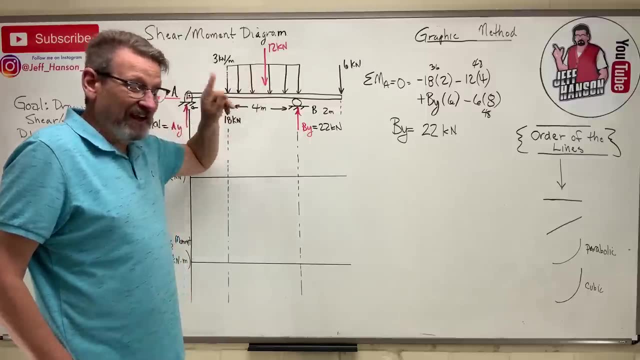 load, because a distributed load plots differently than a concentrated load does. okay, we used a little simplifying technique to find global, but now we got to undo it, we got to get it out of our mind. okay, and the last discontinuity is over, here, at the very end of the beam. 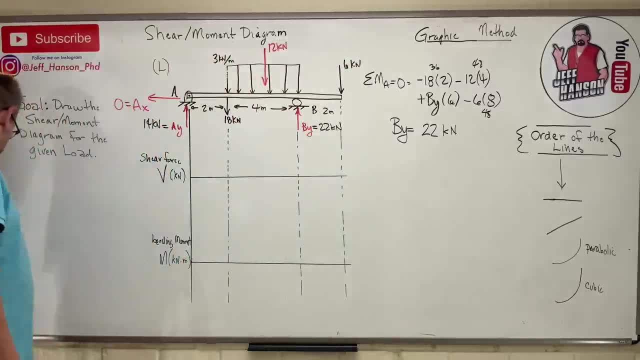 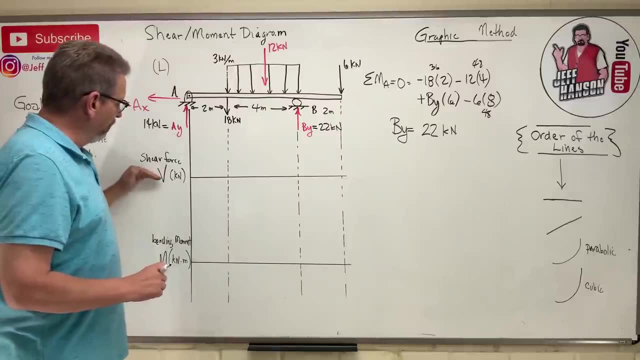 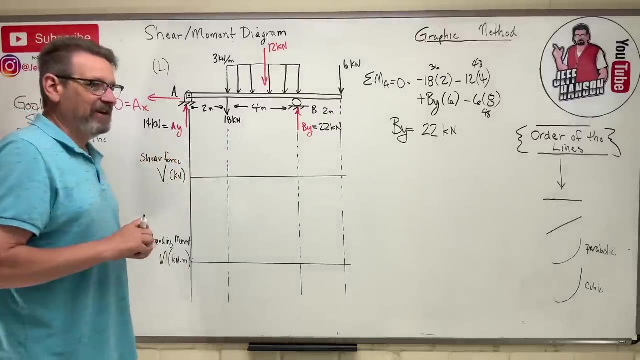 okay. so there's our lines, okay, where i think something interesting is going to happen. okay, now the next thing we're going to. we're going to start here. we're going to plot our v diagram and we'll plot this next, because this one depends on this one, so we got to get this right now. here's. 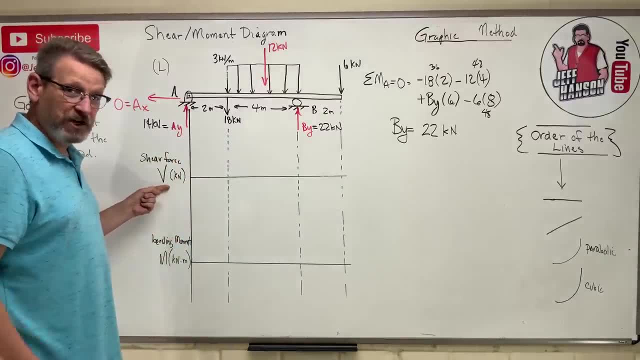 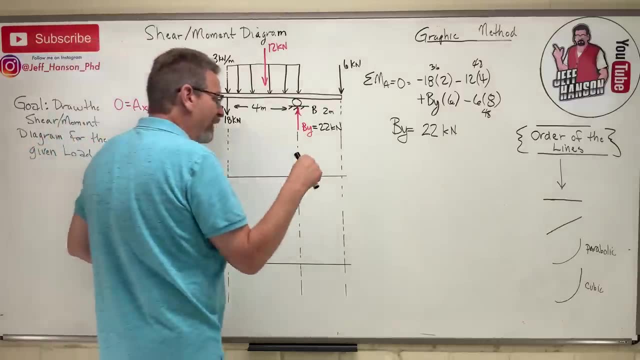 the thing. this is the shear force. so what does this sum of the forces on that beam? zero. so whatever we do here on this graph, we better wind up over here at the end. we better wind up back at zero. if you don't, you've messed something up. 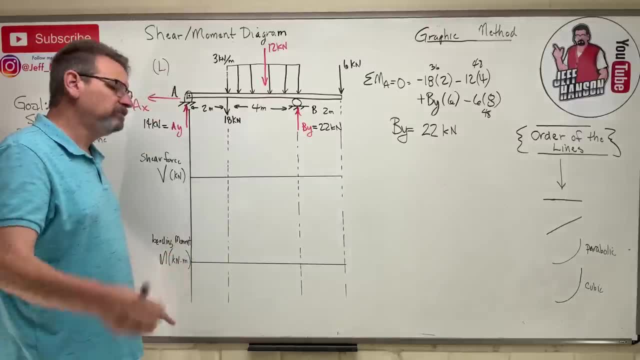 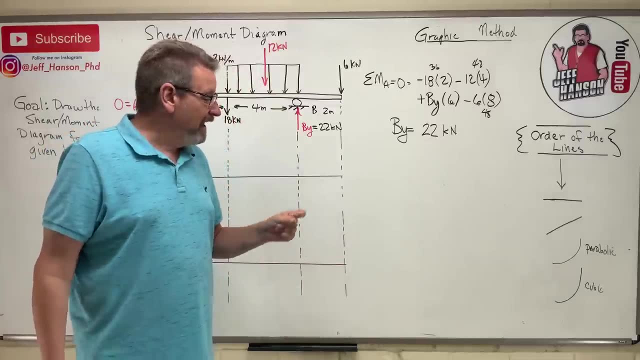 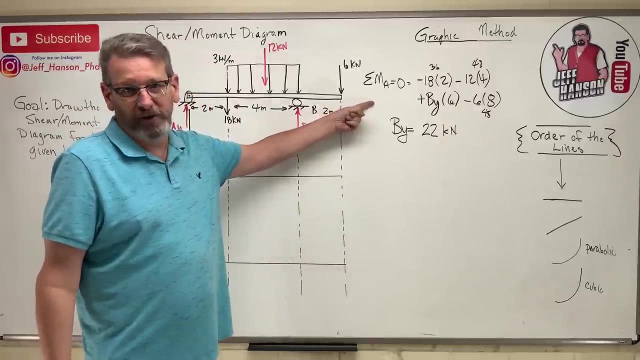 what about m? what is the sum of the moments on a beam? it's zero. so again on this graph, if you don't wind up at zero, you've done something wrong. and if you don't get back to zero on this or this, right then where's the mistake? the mistake is right here. it's a global equilibrium. it almost always. 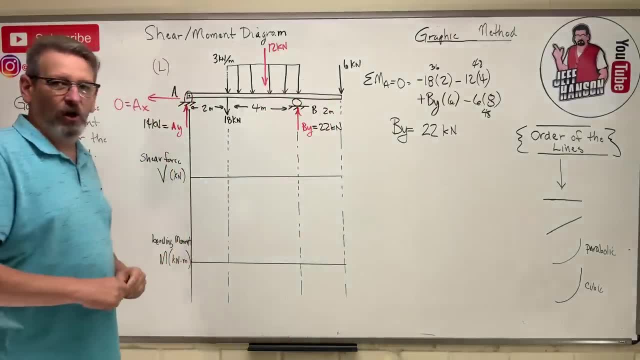 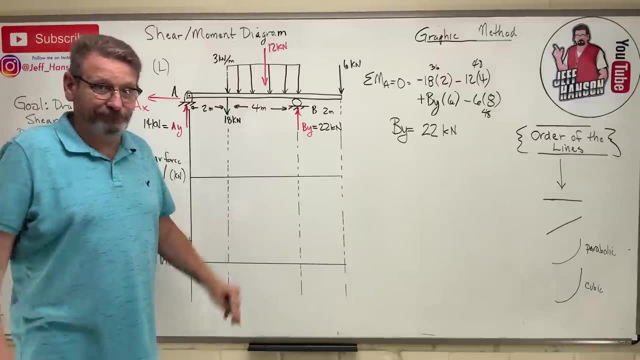 is global equilibrium. okay, go back and check your global. so that's the nice thing. you shouldn't miss these problems, because you wind up back at zero and if you don't, then you're like, well, something's not right. okay, it needs to wind up at zero, all right. so imagine this. I'm fixing to get on this. 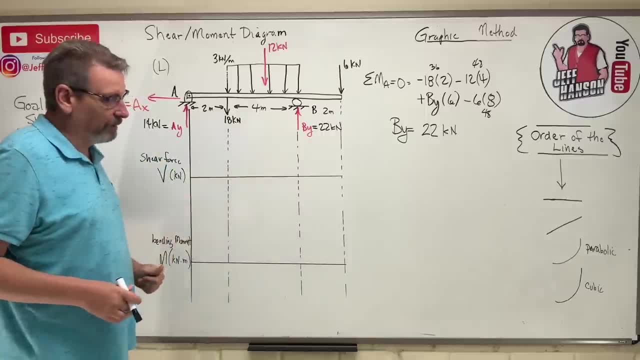 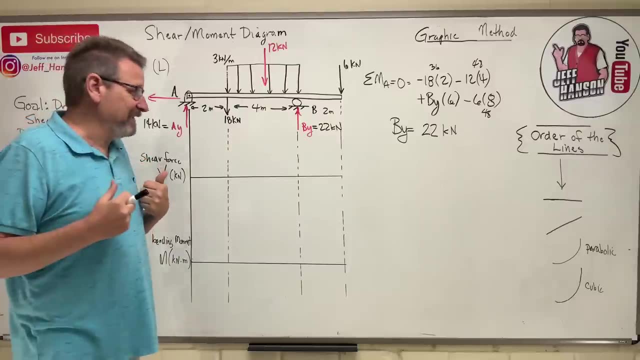 beam and I'm going to walk across it from the left to the right. okay, I'm going to hop up here and start walking across it, okay, but I got me a load backpack on. I got my backpack on. it's completely empty. as I go across this beam, people are going to be putting things in my backpack, right that's. 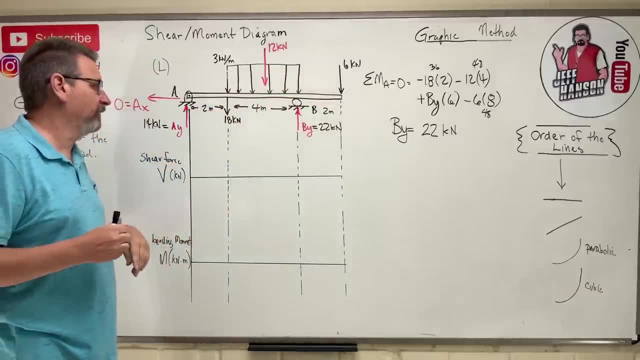 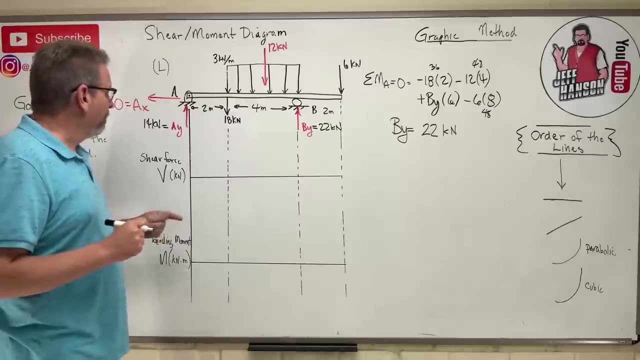 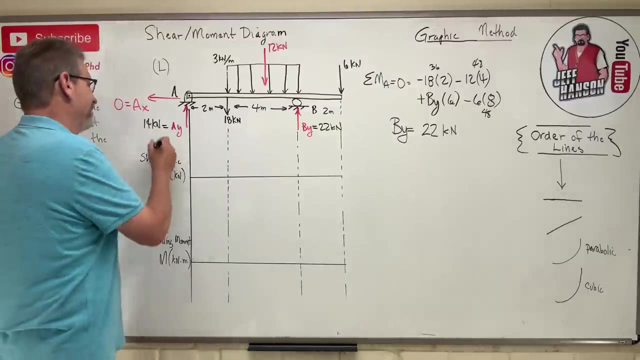 these loads that I that I'm going to incur across this, uh, beam as I go, as I go along. so let's see if we can graph the v diagram. all right, here we go, we hop on the beam. the first thing we get in our backpack, bam, 14 kilonewtons up. that's a, that's a van halen force right there. 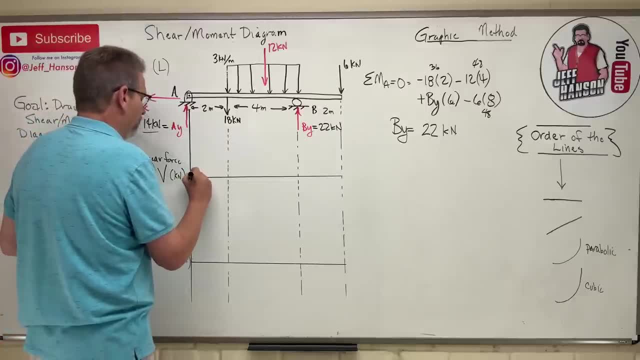 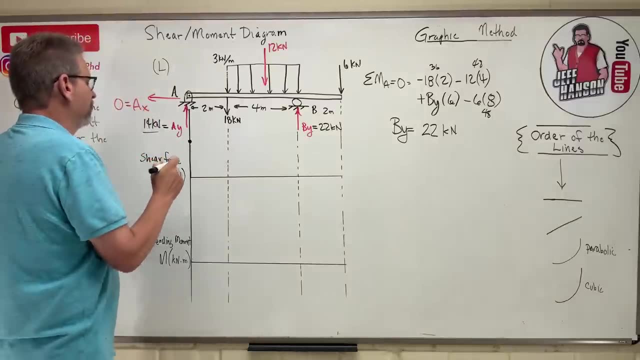 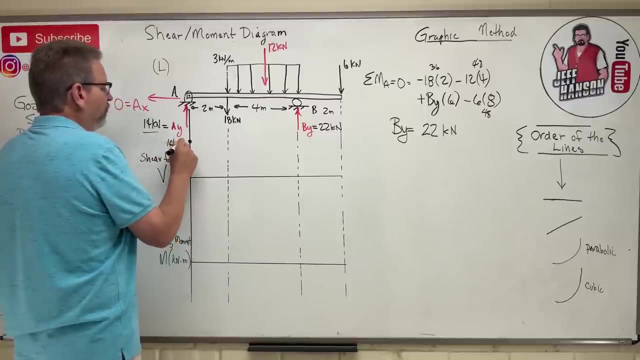 my. might as well jump. go ahead and jump. I hope. I hope they don't get me. youtube will find me for using music, right? maybe it won't recognize it? uh, probably not. okay. so here we go: 14 kilonewtons. that's where we are, and we don't have to put the units on these, because we we have the units on our. 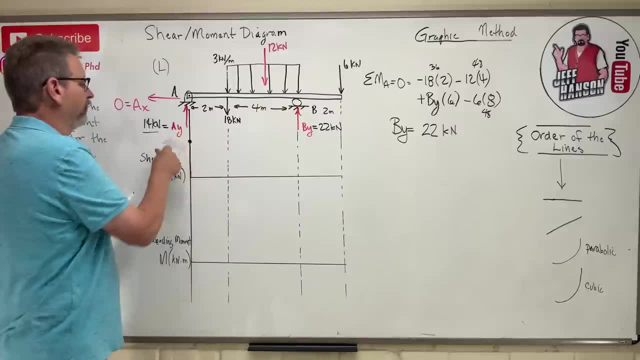 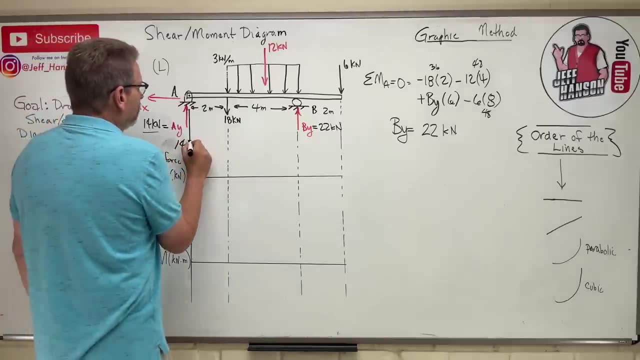 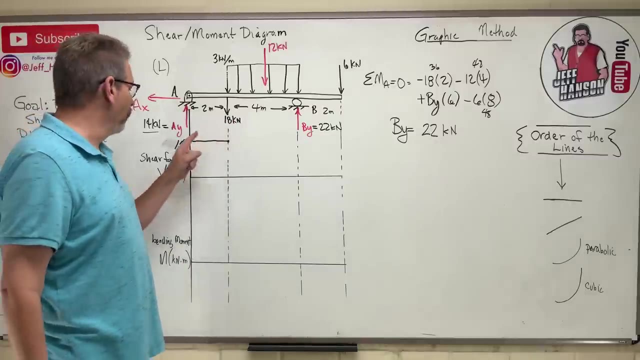 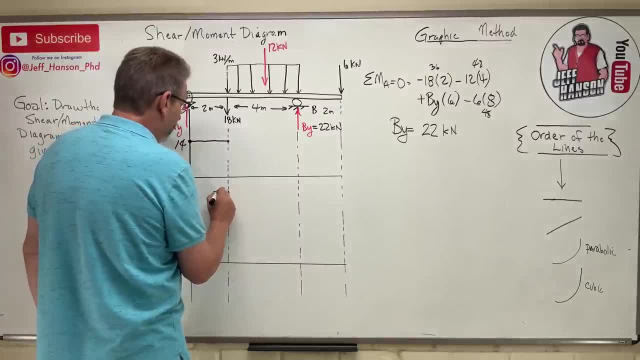 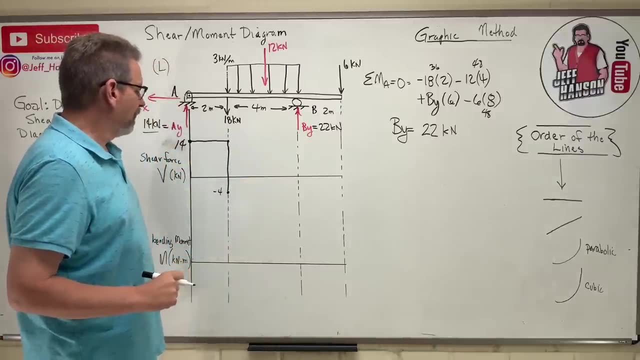 where am I now? whoop, I'm at negative four. okay, whoop, straight down. bam, another one made me jump, didn't it all? right now, from there, I've got to go down 12 more. and how do I go down 12? well, I take a. 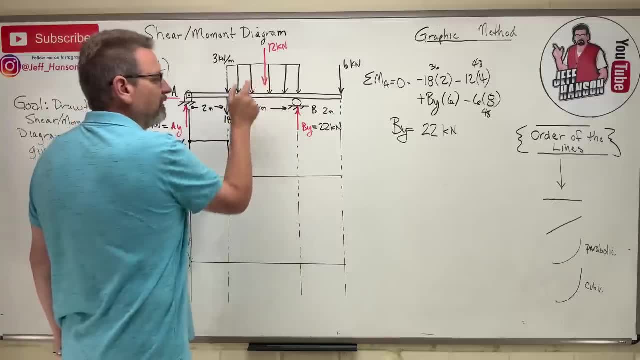 get three. Take another step: I get three more. Another step: I get three more. So I'm going down, down, down, down. That's why it's a straight slope. So I'm at four By the time I get over there. 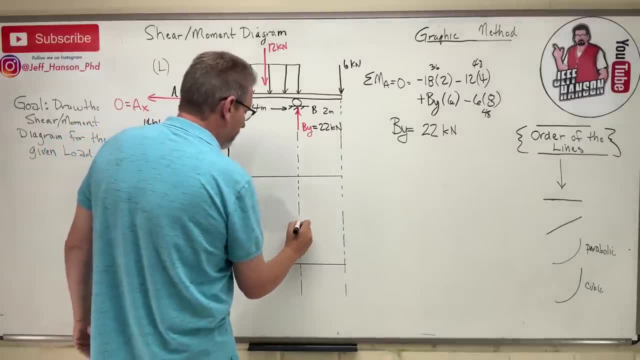 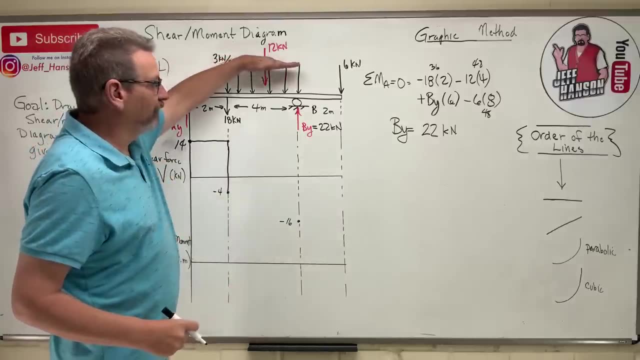 I'm going to go down 12 more, So I'm going to be at bam negative 16.. And how do I get from there to there? Again, I've got a straight across line, So the next graph down has to be a straight slope. 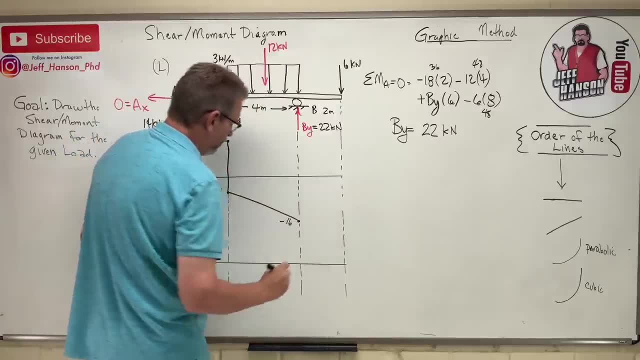 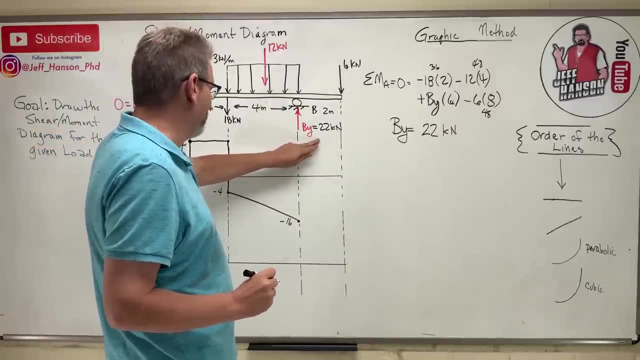 right. So like this, That's pretty straight. Now what happens? Bam sick Got another jump here, 22.. Well, that's going to take me 22.. Let's see, That's going to take me up here to positive six. 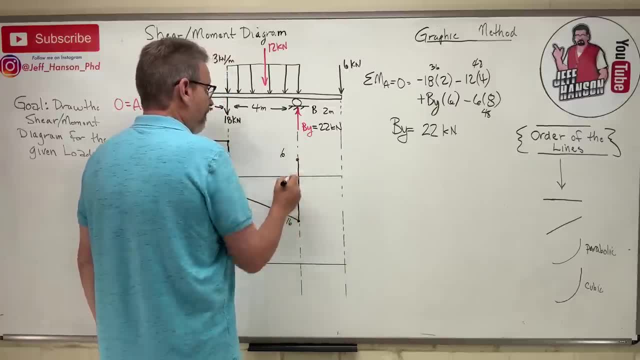 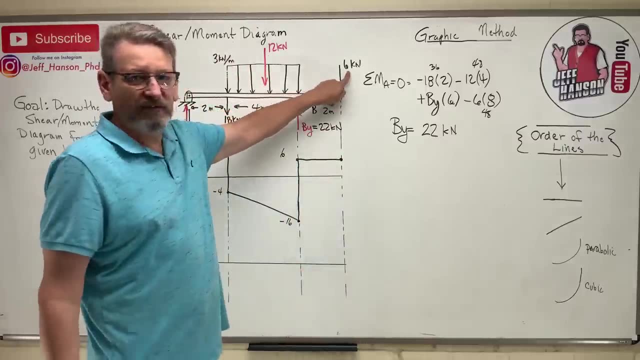 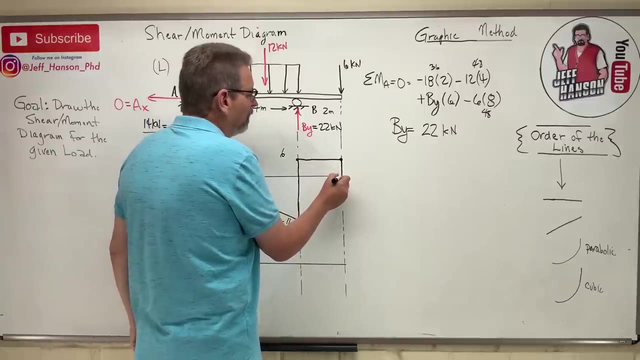 So here we go. Okay, Let's walk some more. No change, no change, no change. Bam into the beam. John Denver force. Take me home, Home, to the place I belong on my shear graph Back to zero. There you go. That's too silly. 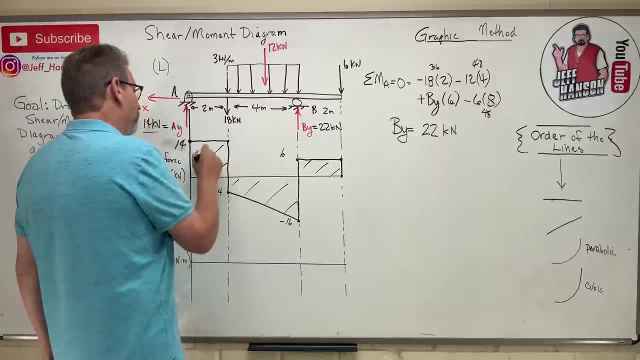 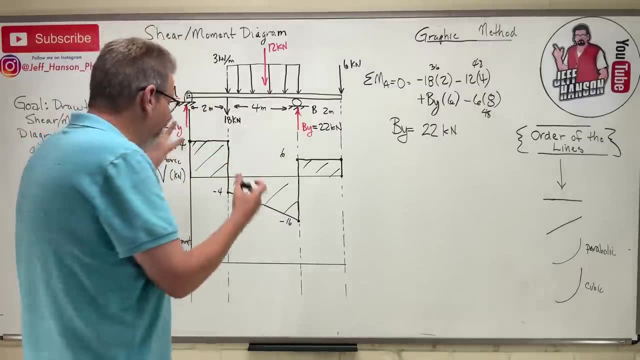 You're so silly. Hey man, if it helps you remember how to do these graphs, then I'll sing to you. I don't care. Okay, So we got our V diagram, That's it. So if I ask you, what is the biggest shear? 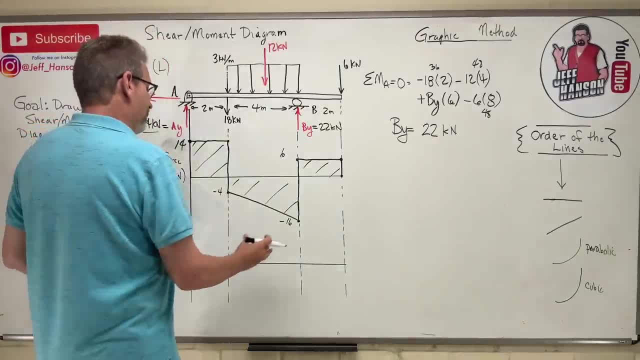 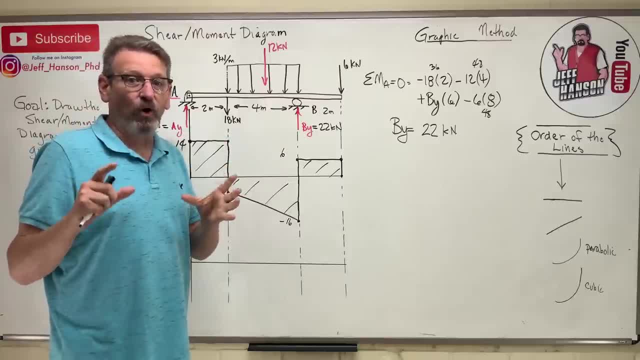 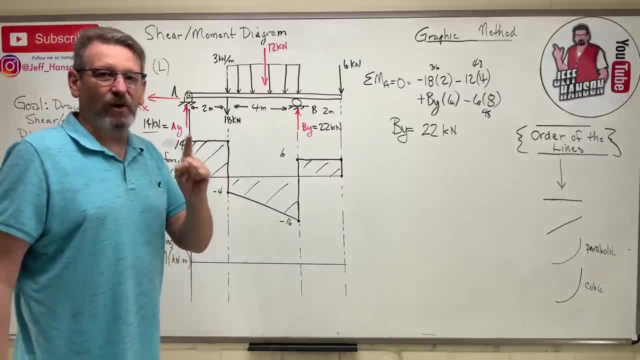 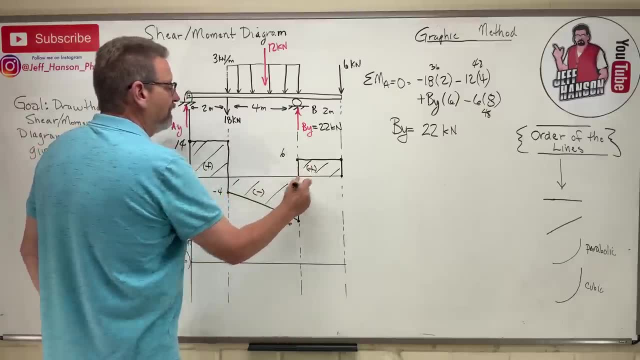 it's 16.. Okay, So the next thing I do on this is I put me some little pluses and minuses. Okay, Plus, minus, plus. Okay. Anything above the line gets a plus, Anything below the line gets a. 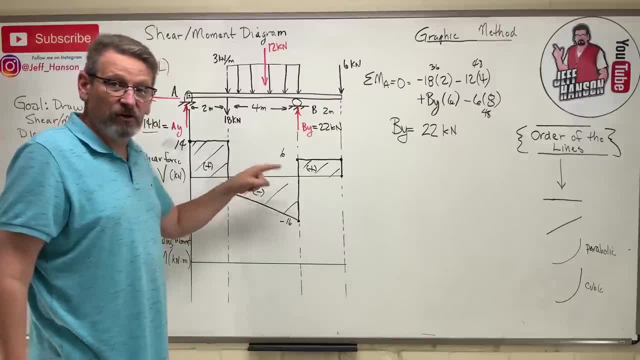 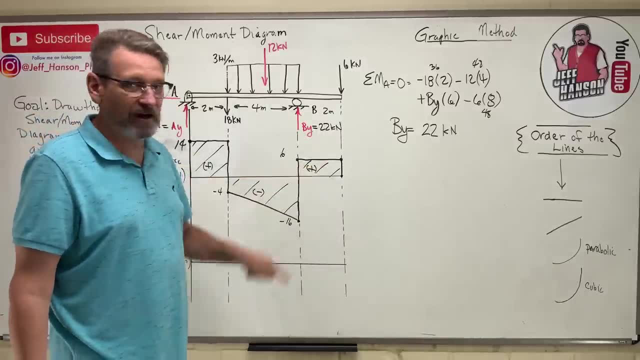 negative, And that tells me what the slope is going to do on this next line down here. Okay, So that tells me that my M diagram is going to go uphill, downhill, uphill. okay, so that's what that slope is now. here's where the graphic method. 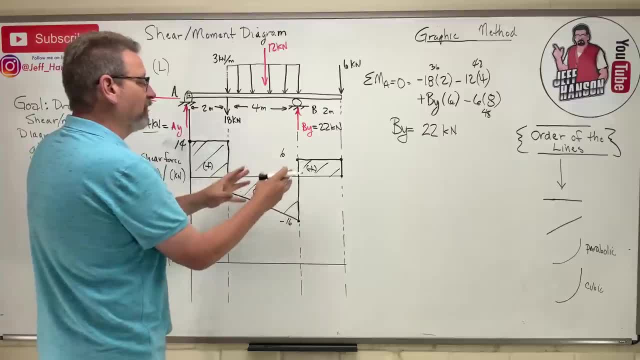 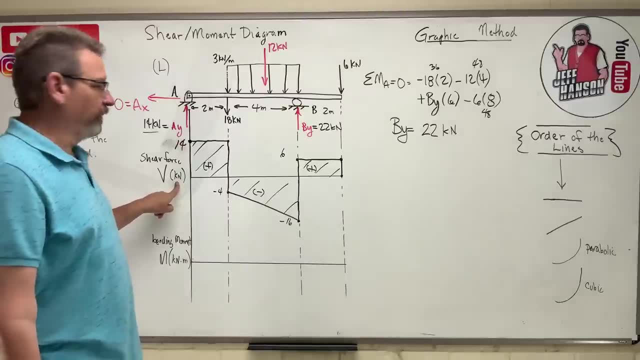 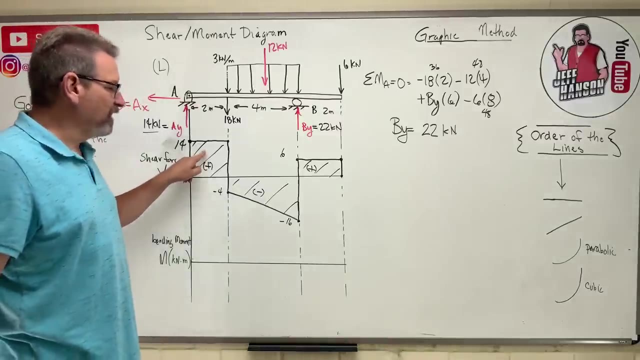 comes in into play. we're going to look at these shapes that we made here. okay, because the height of these shapes are in what? the height is in kilonewtons, and the width of these shapes is in meters. so if I find the area of that shape, it 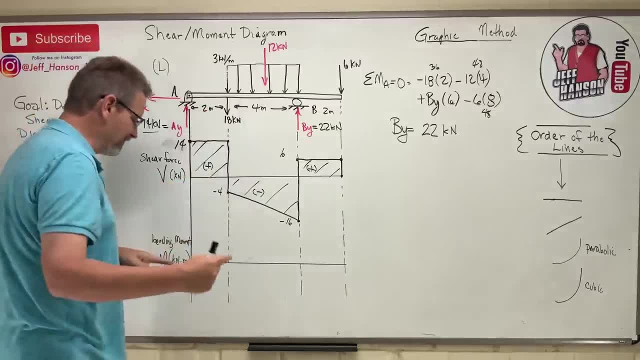 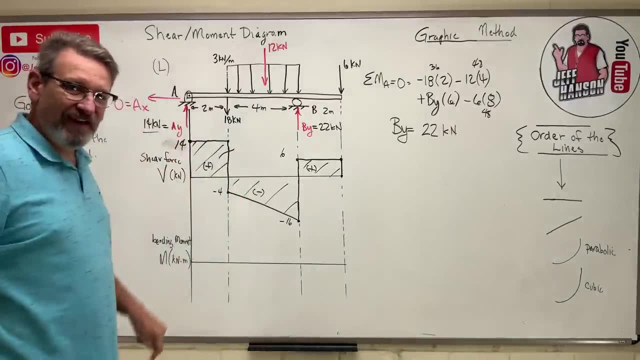 would be height times width, which is kilonewton meters, which is a moment. so the area of these shapes gives me the moment that I'm going to use on that next graph, okay, so I like to do these and put a little circle around them, for 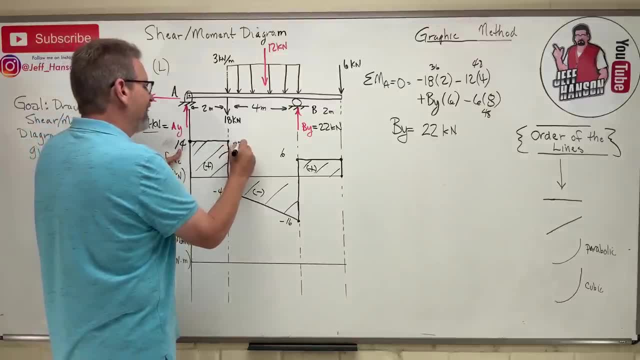 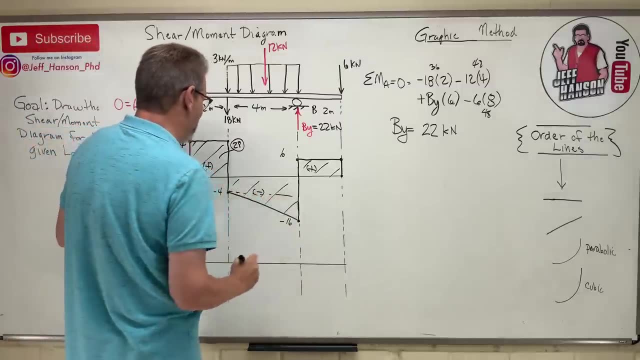 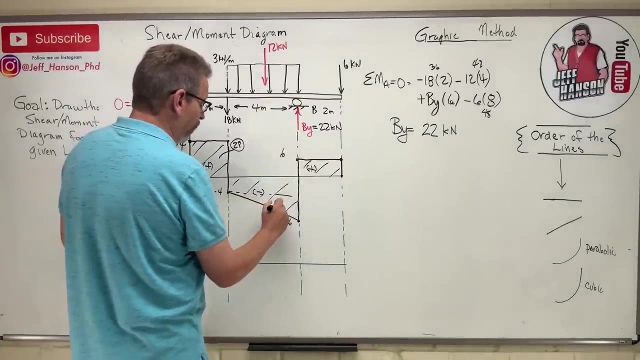 instance, this is 2 times 14, so this area is 28. so I put a little circle around it that tells me that that's his area. now this guy is made up of a rectangle and a triangle. right the triangle is 4 times 12, is 48. divided by 2 is 24, that's 24, and 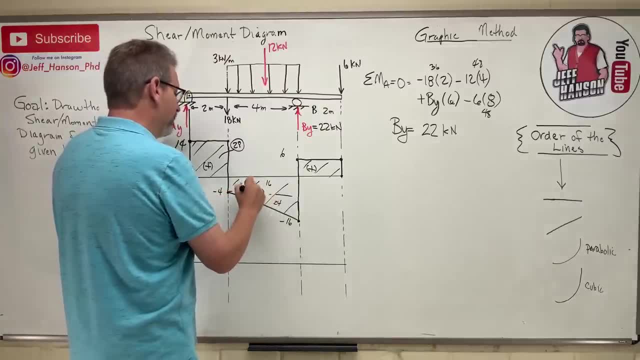 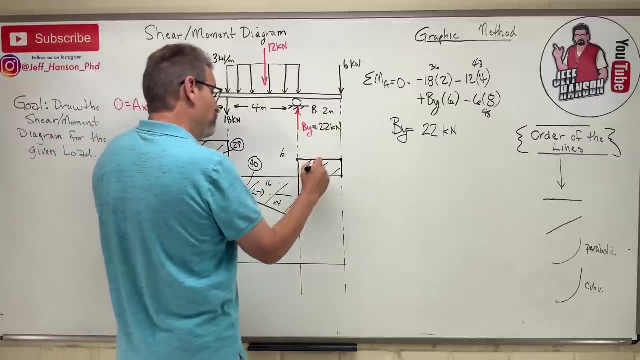 this part here is 4 times 4 is 16. so the area of this guy is 40, okay, and then finally, the area over here is what? 6 times 2, 12? okay, so there's my areas. I'm ready to do my moment diagram now. 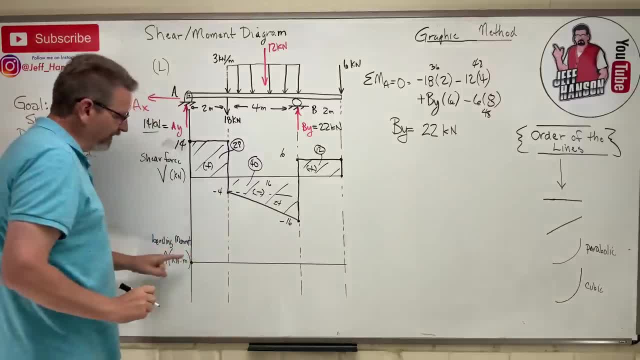 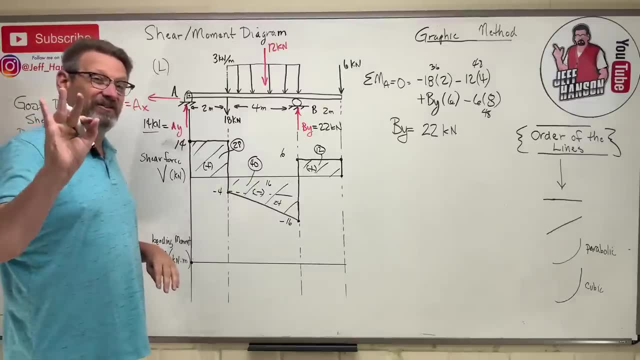 okay, so here I am. I'm starting at 0. the only time you don't start at 0 is if you have a concentrated moment here and you can watch the next video and I'll show you how to deal with concentrated moments. really a nice trick. another: 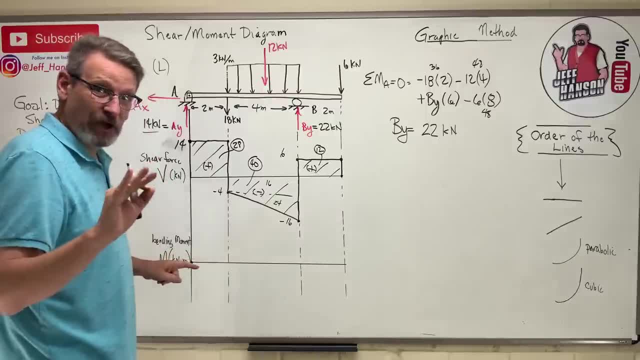 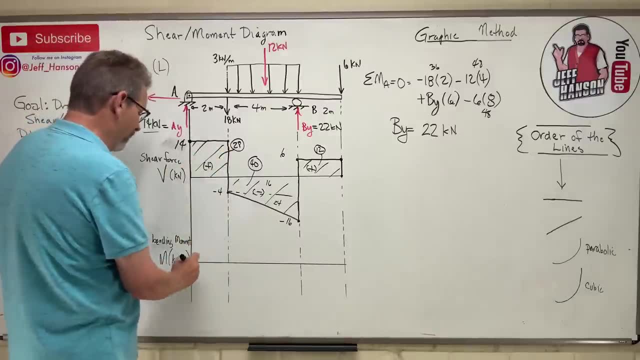 little saying for you to remember in the next video. it's a treat you gotta go see, okay. so here we go. we're starting off at 0. we're gonna go uphill. how much 28? okay, we go to 0, we go to 28. there's 28 right there. 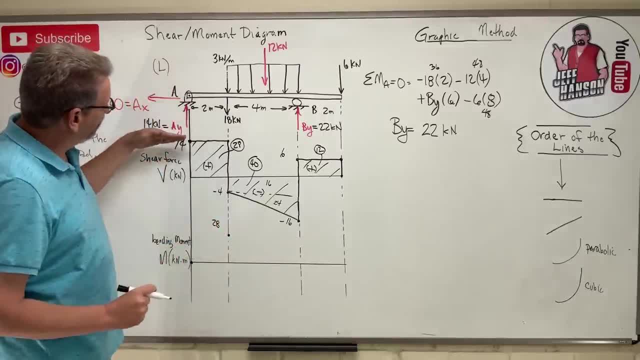 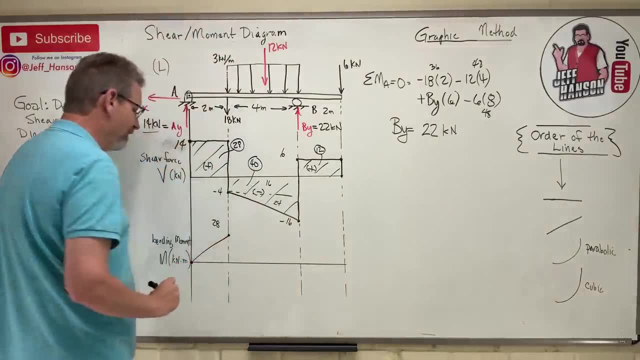 how do I get from there to there? well, let's see that one was straight across, so the next one is gonna be straight slope. oh, this is not hard, is it okay? bam, then I got to go downhill. 40. I'm at 28. that's gonna take me to negative carry. 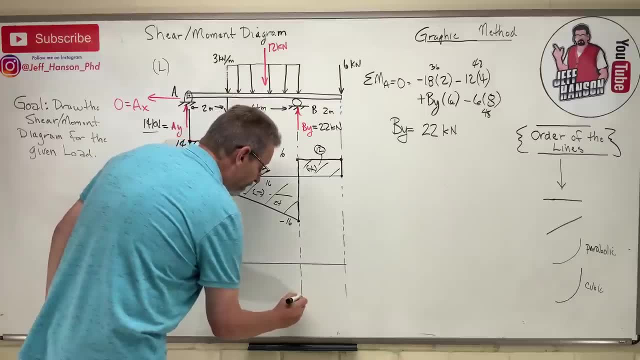 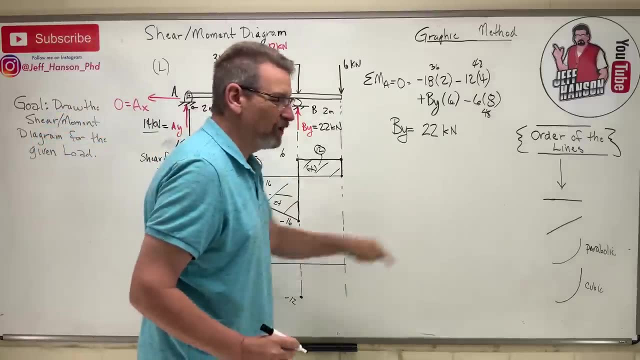 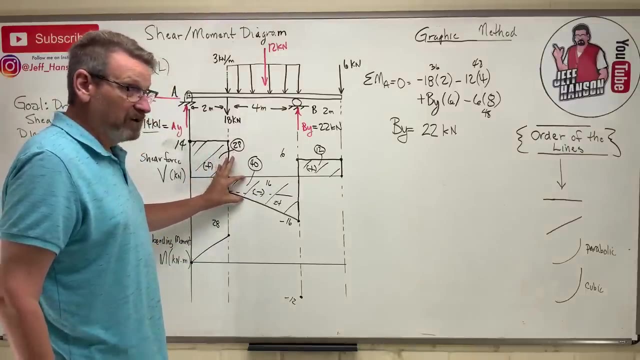 the 9. okay, so here I am. negative 12. how do I get there? oh, oh, oh. oh, this one is a slopey do. the next line down is gonna be parabolic. why is it parabolic? well, I'll take a step over here. I get 4. then the next step: I get something more than 4. 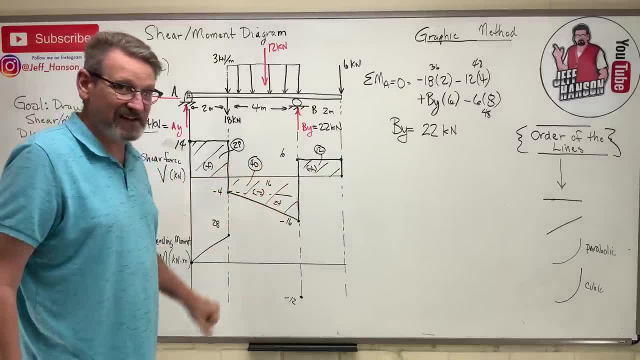 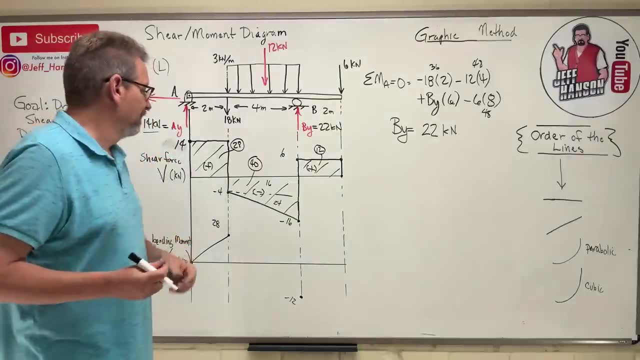 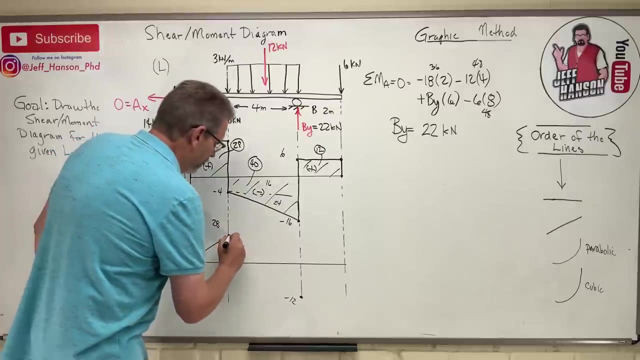 and then something more than that, and then more, and then over here I get 16 right. so I'm not accumulating load linearly, I'm accumulating it parabolically, and so what? here's what we do. I have to go from here to there. so I'm gonna give you two choices: okay, and that's this, or 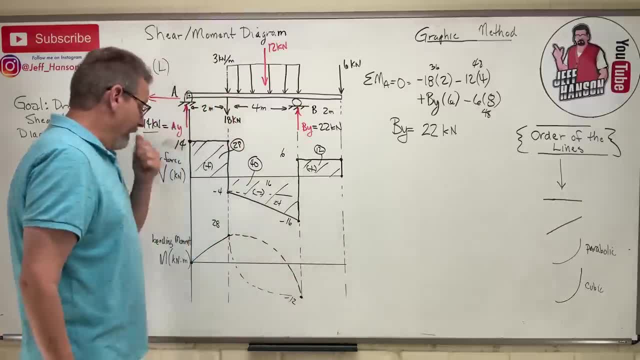 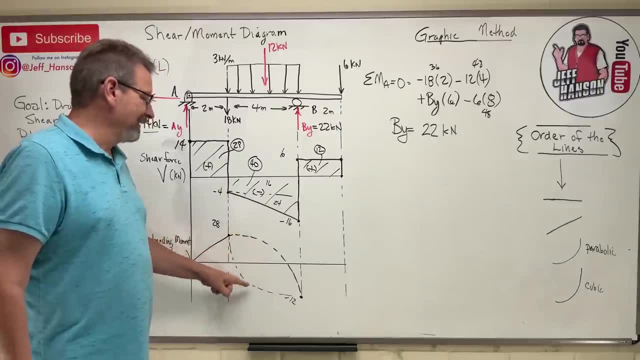 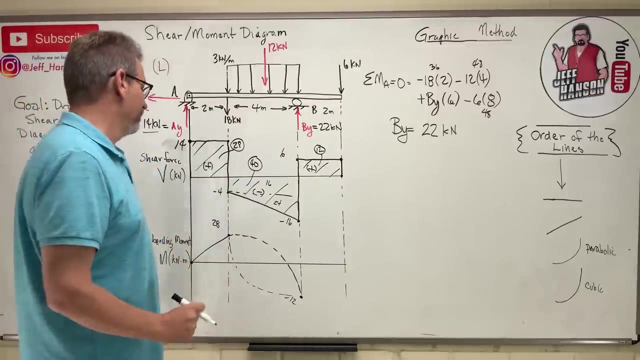 this. okay. now, this is the number one mistake students make is choosing this inflection here, wrong or incorrectly. okay, but I'm gonna teach you a little trick that gets it right every single time. and it goes like this: okay, I take a step over here and what? avoid it? short stack. well now, if I take that same step compared to this another one I take, and what we get? short stack, and that's what's happening again and you're not exactly looking liking the same thing. well, now you're not actually using these steps when they goЖak or I門 counties System. 아喔, Master, Uruguay.